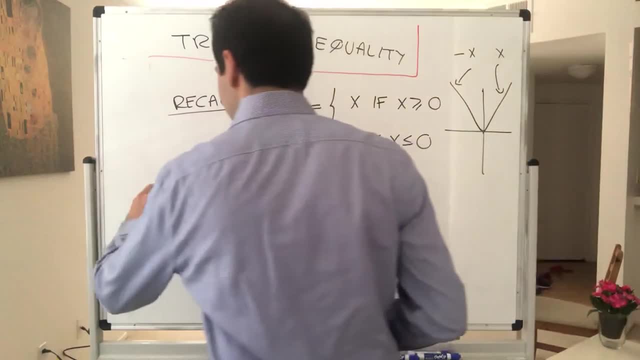 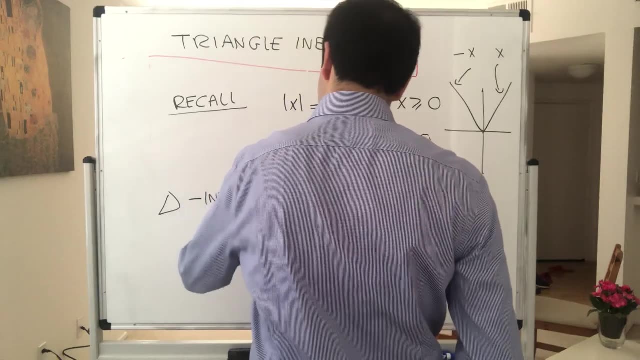 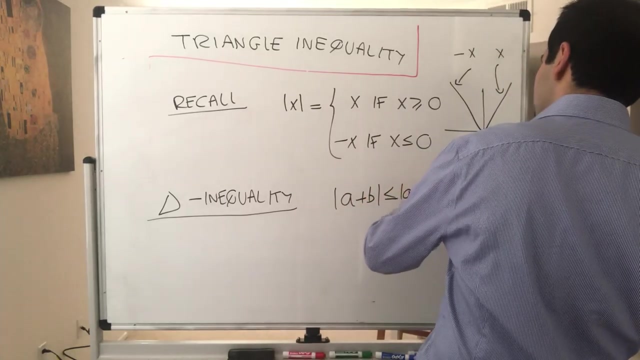 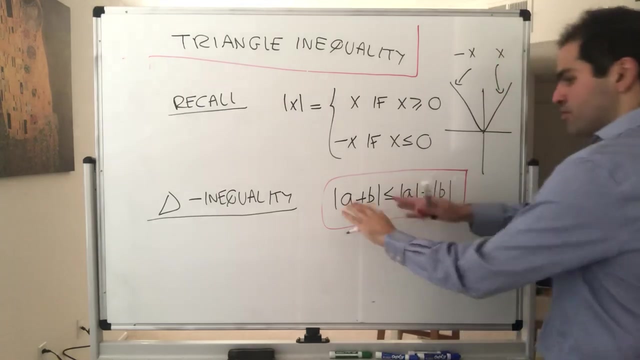 times absolute value of b. But, most importantly, you can prove, state and prove the triangle inequality, which simply says that the absolute value of a plus b is less than or equal to the absolute value of a plus the absolute value of b. So it's almost like just taking the absolute values out. 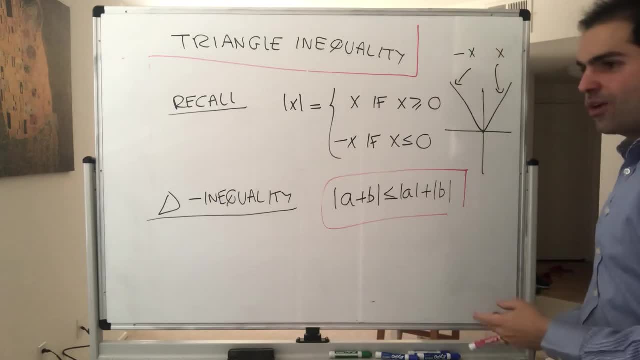 but it's important that you have to have the inequality, And I'll explain in a second about why this is so important. So I'll explain in a second about why this is so important. So I'll explain in a second about why this is so useful. 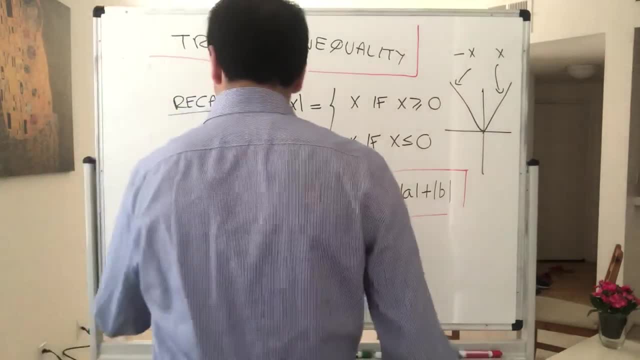 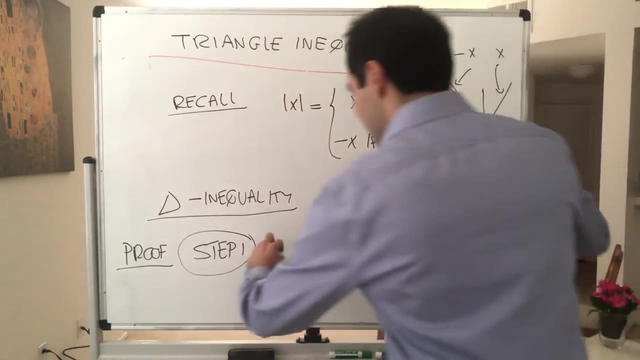 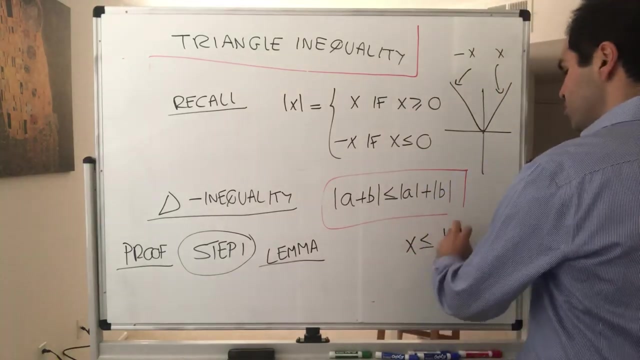 But first let me prove this, And first we just need a small lemma which may or may not be obvious to you, but let me still state it: Namely, x is always less than or equal to its absolute value, and it's always greater or equal to negative. 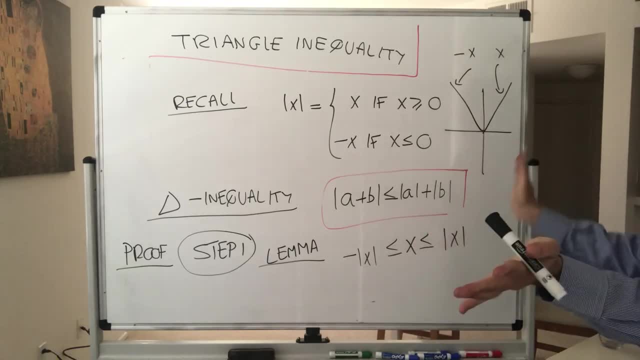 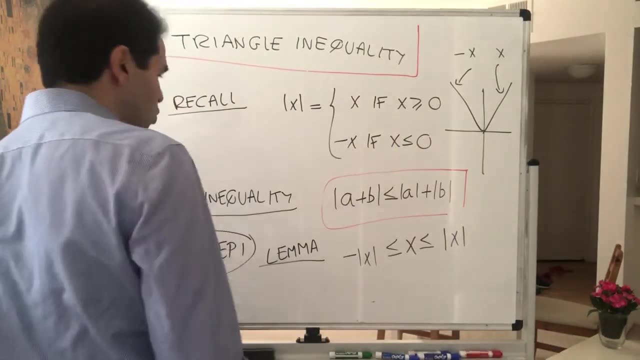 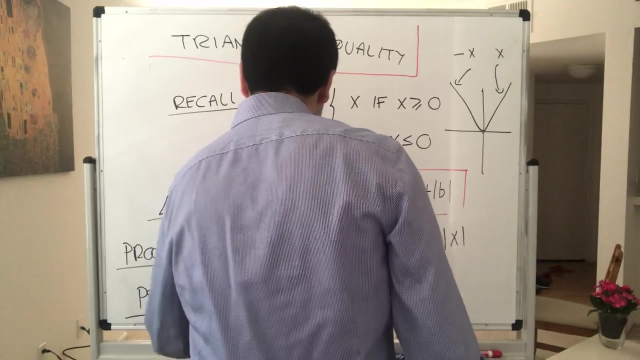 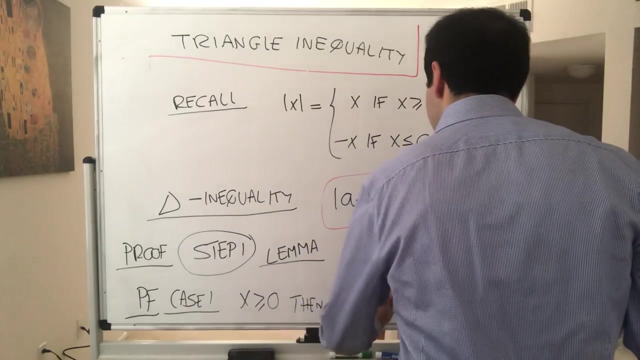 its absolute value. So x is always squeezed between its magnitude and negative its magnitude. And why is that true? Well, just consider two cases. So if x is positive, then well, x equals to its absolute value, and therefore x is less than or equal to its absolute value. 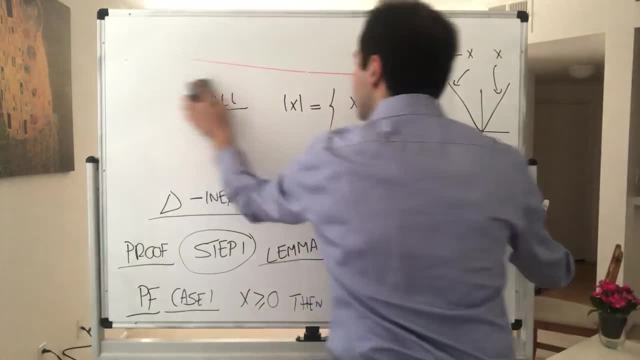 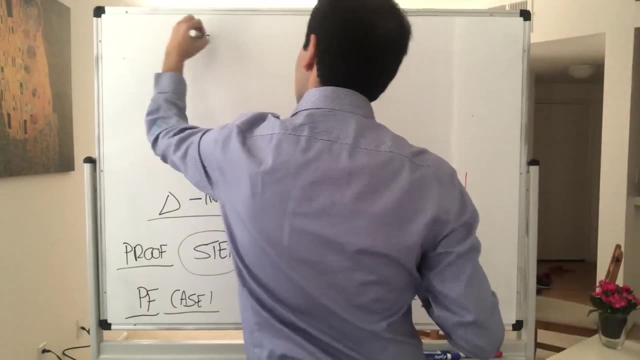 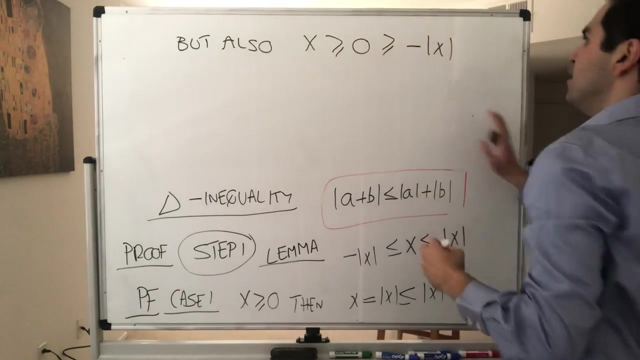 On the other hand, since x is positive but minus the absolute value is negative. On the other hand, since x is positive but minus the absolute value is negative, we also get the other side: x is positive and that's less than or equal to minus. 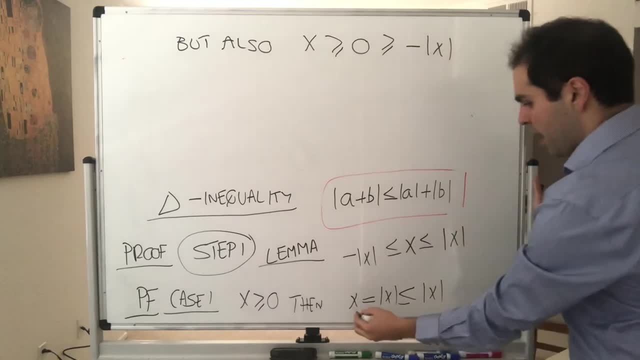 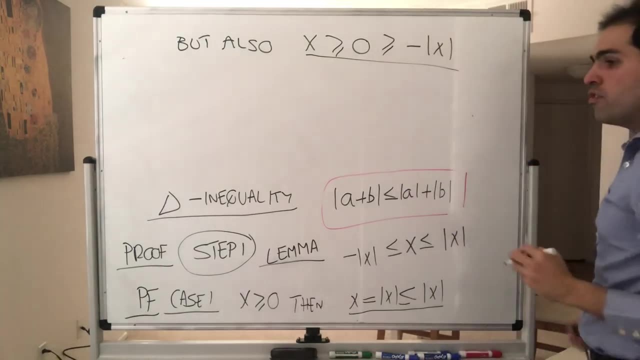 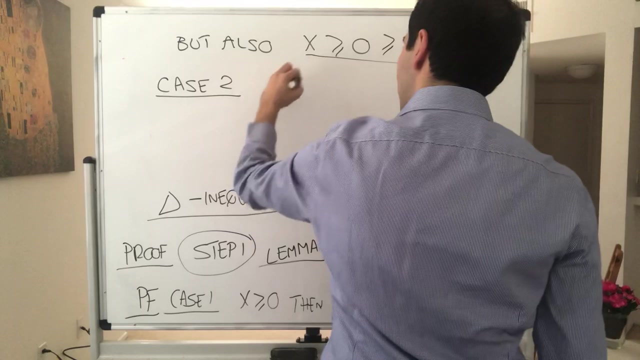 the absolute value of x, because this is for sure negative. And then you just combine that. So x is less than or equal to its absolute value, but x is also greater or equal to its negative absolute value. And now case two. Well, if x is negative, 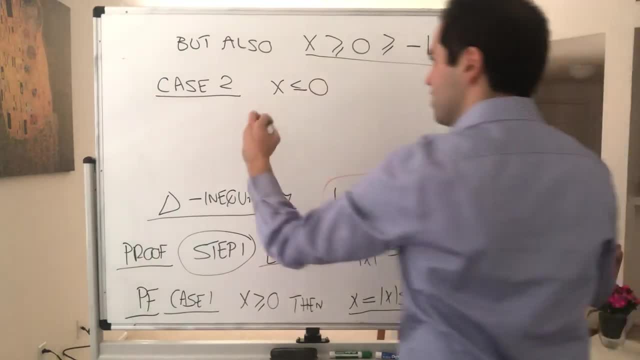 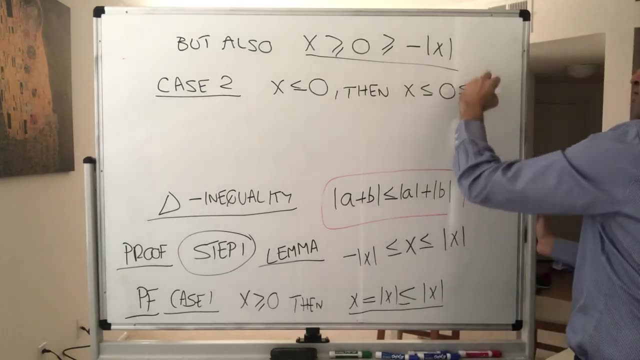 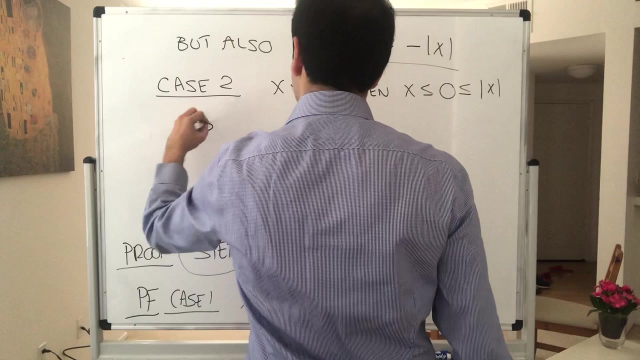 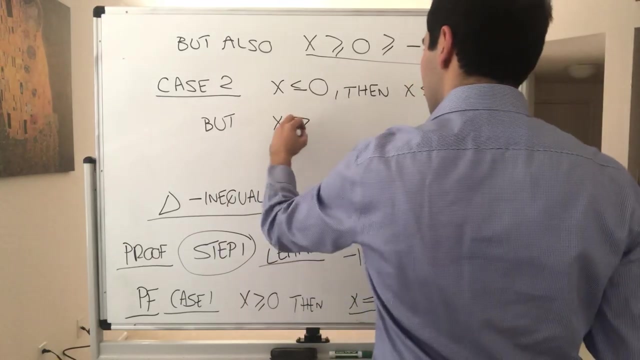 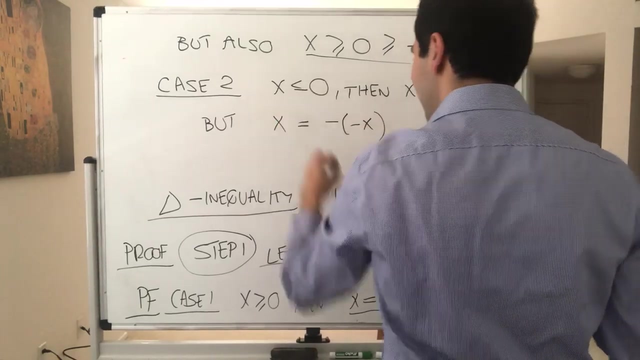 then, since the absolute value is positive, first of all, x, of course, is less than or equal to its absolute value, But also, well, x is also well greater or equal, I think, to minus minus x. Well, x is equal to minus minus x. 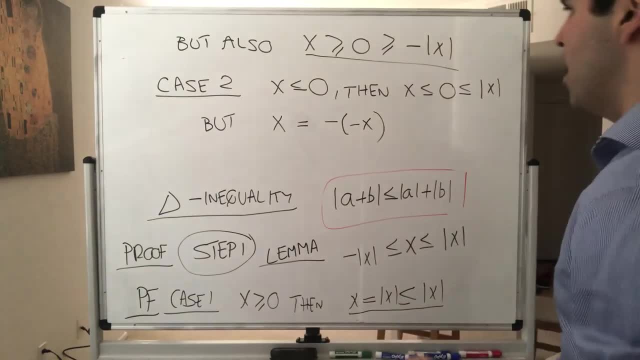 but also minus x. in this case it's minus the absolute value of x. Minus x is the absolute value of x. So in other words, we also get in particular, that x is greater or equal to minus the absolute value of x. 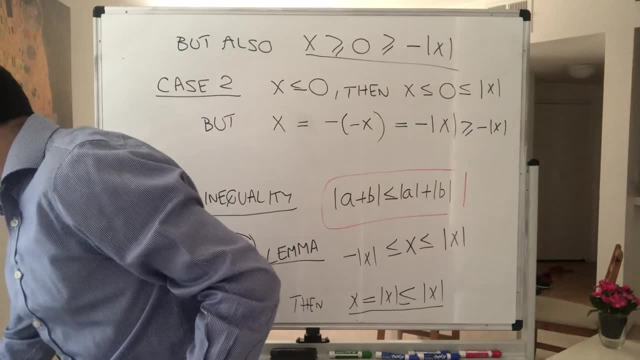 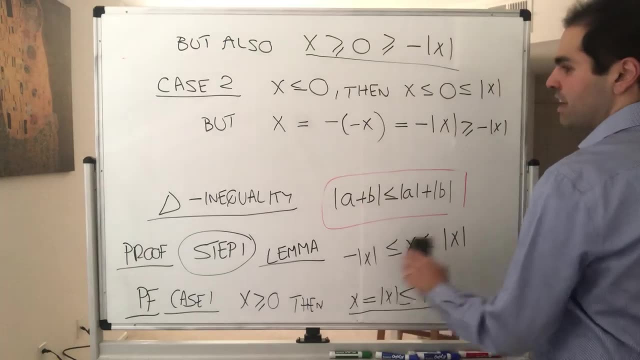 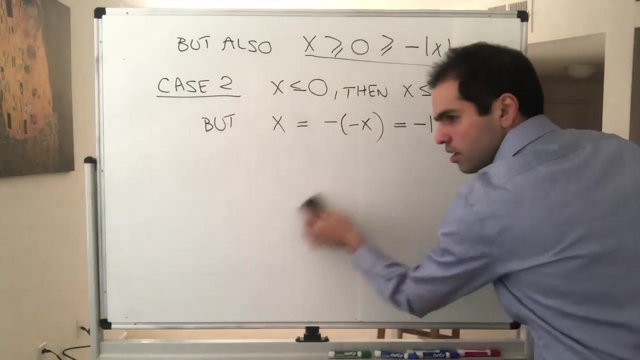 because it's equal in this case. All right, Okay, now how do we do this? Again, it's very important. x is squeezed between its magnitude and negative its magnitude, And then all we need to do is just consider again, play around with this a little bit. 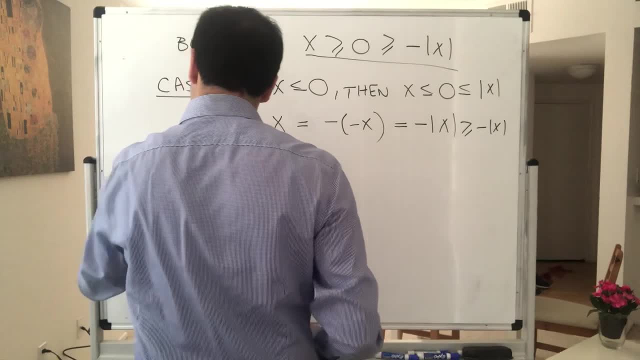 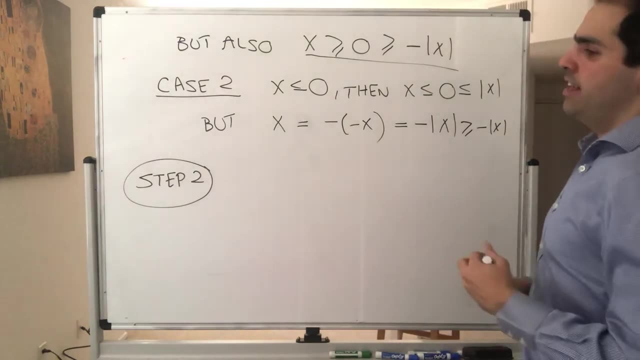 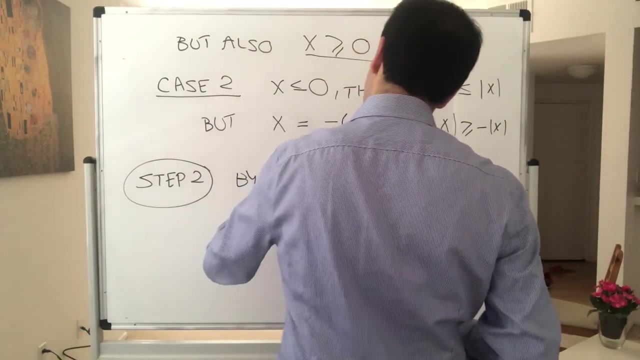 So step two. So, again by dilemma, again we want to show that absolute value of a plus b is less than or equal to absolute value of a plus absolute value of b. So by dilemma, again, we know that a it's squeezed between absolute value of a. 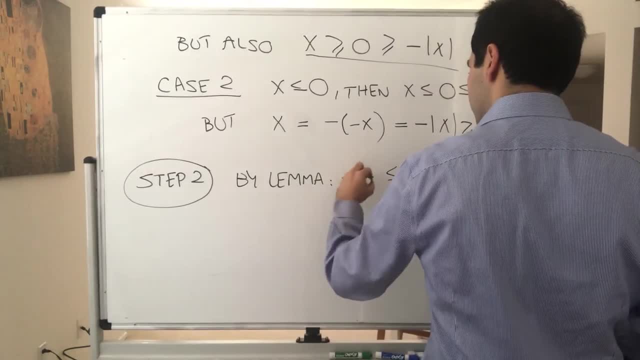 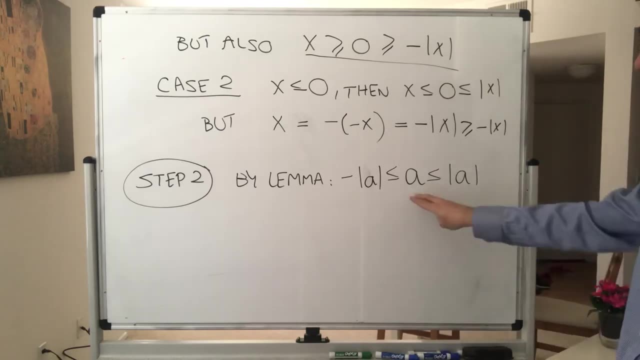 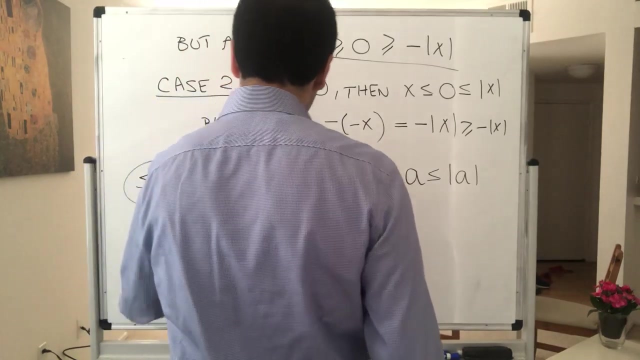 and minus absolute value of a. Well, and then here's a trick. So we want ideally absolute value of a plus b, So let's add b to both sides, So a less than or equal to absolute value of a. Well, that implies a plus b is less than or equal. 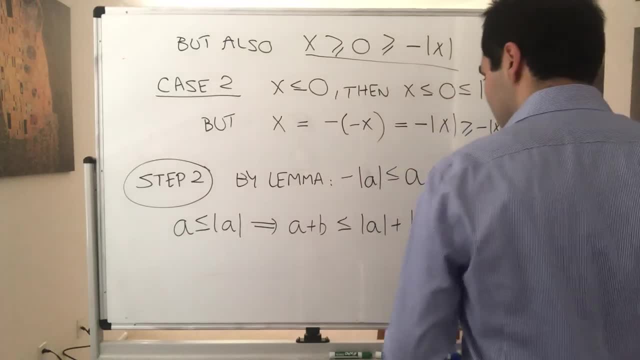 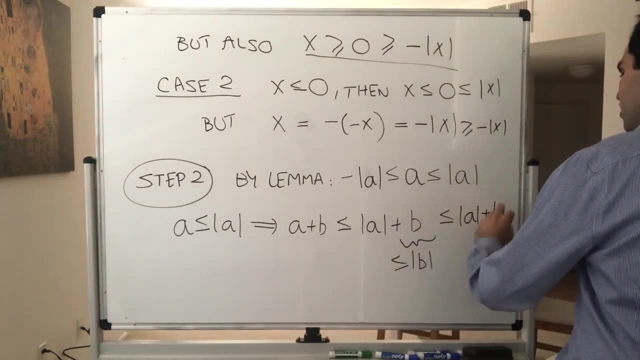 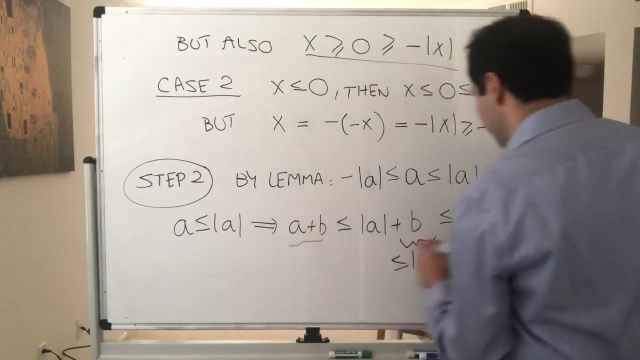 to absolute value of a. So a plus b. But remember, b is also less than or equal to its absolute value. So this is less than or equal to absolute value of a plus absolute value of b. So that's good. a plus b is less than or equal to the absolute value. 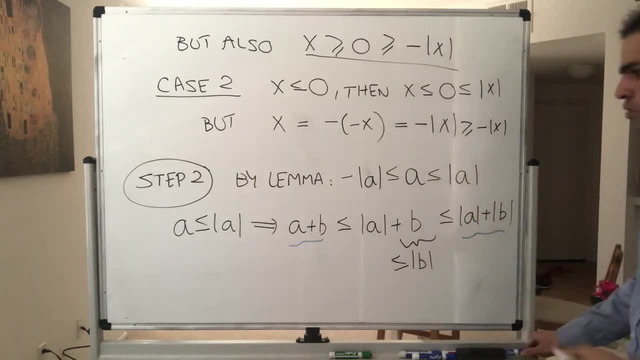 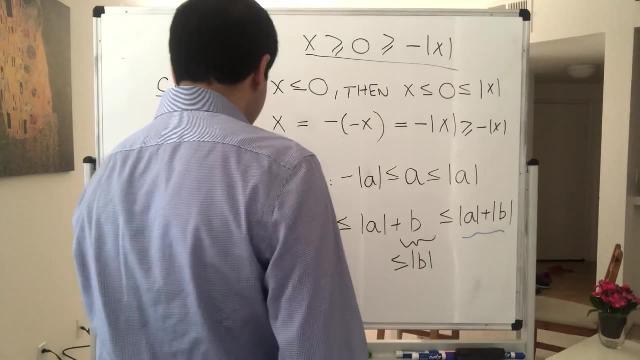 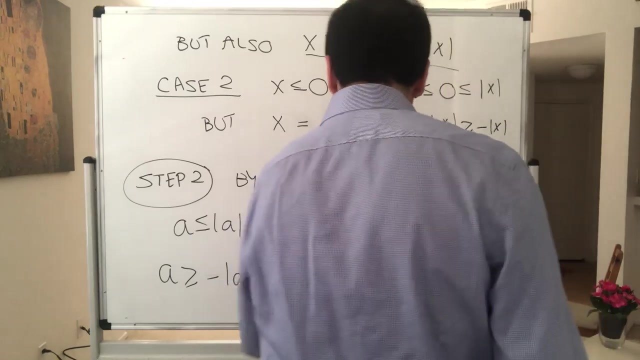 of a plus the absolute value of b. And now we want to do the reverse. So a is greater or equal to minus absolute value of a. And so a plus b is greater or equal to b minus absolute value of a. but remember, b is less greater or 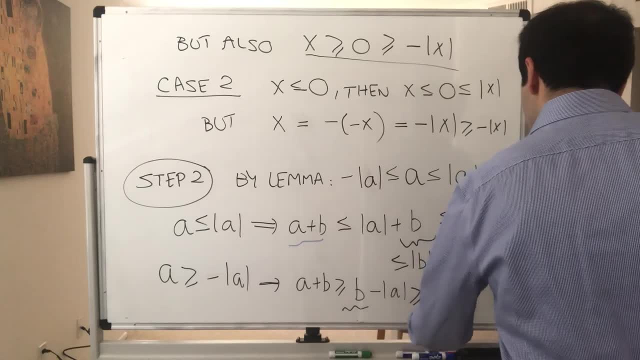 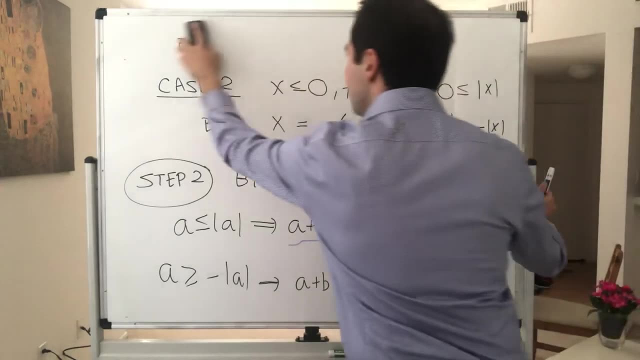 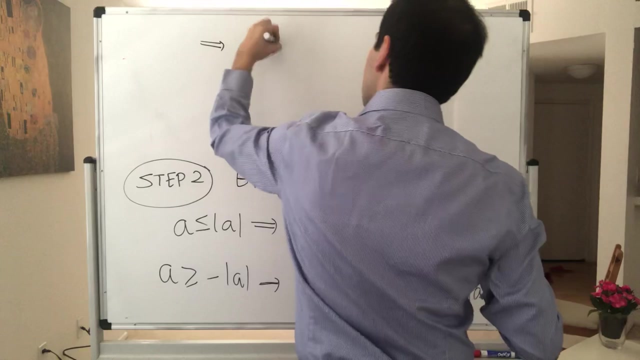 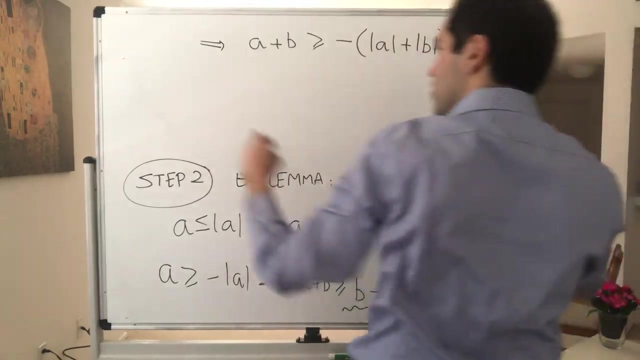 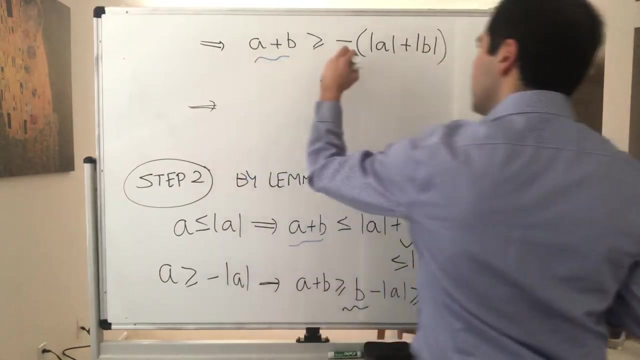 equal to minus absolute value of b. so, indeed, what we get is that a plus b is greater or equal to minus, is greater or equal to minus absolute value of a plus absolute value of b, and so, in the end, if we combine both things, we get that a plus b is actually squeezed. 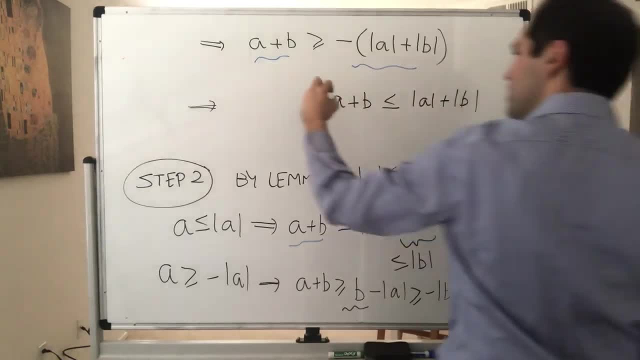 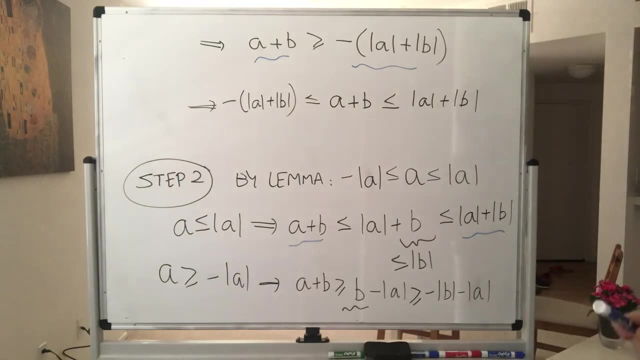 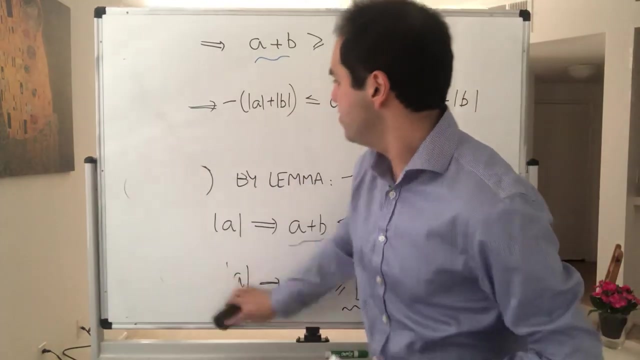 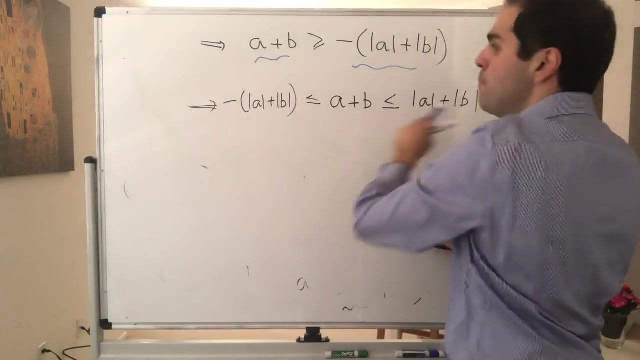 between absolute value of a plus absolute value of b and minus absolute value of a plus absolute value of b. so in particular again next step, either obvious or not obvious to you, i mean not quite obvious for me- but if a number is squeezed between two positive numbers, so m and minus m. 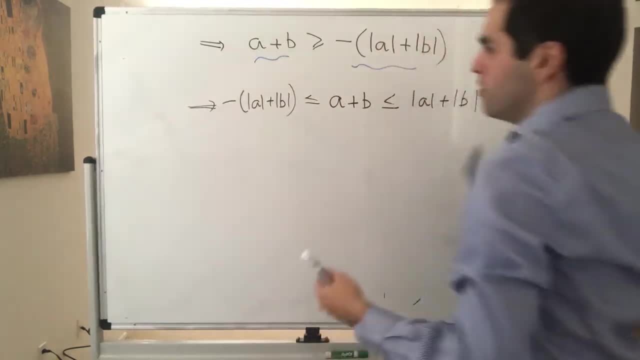 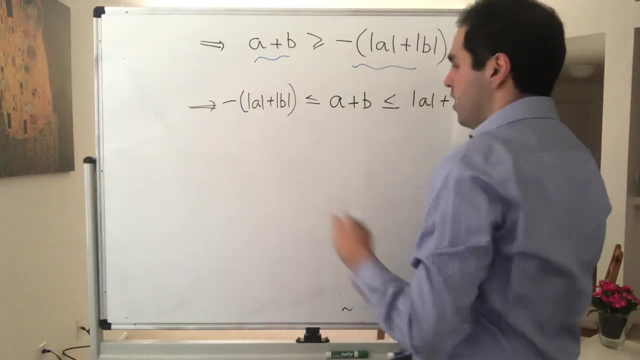 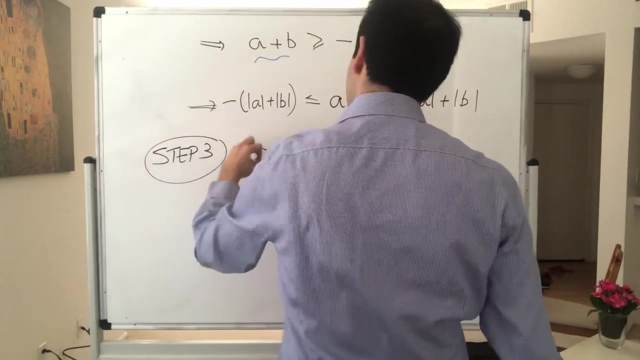 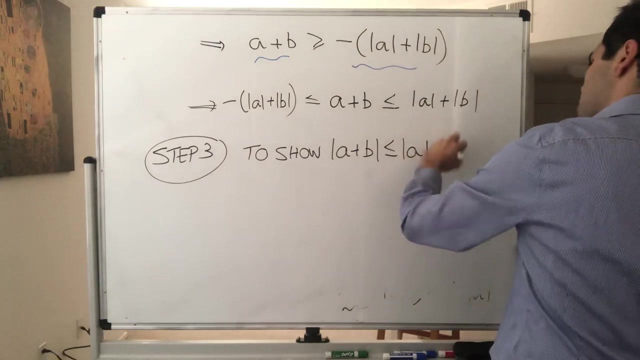 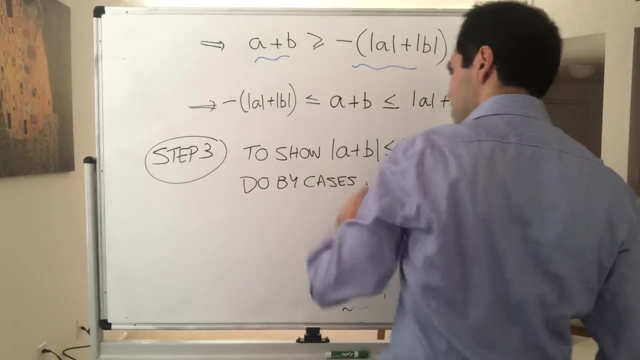 then the absolute value of that number is less or equal to m. but as i said, for me it's not quite obvious, so let me just prove this again by cases. and lastly, to show our result, do it by cases. so case one: assume this is positive. 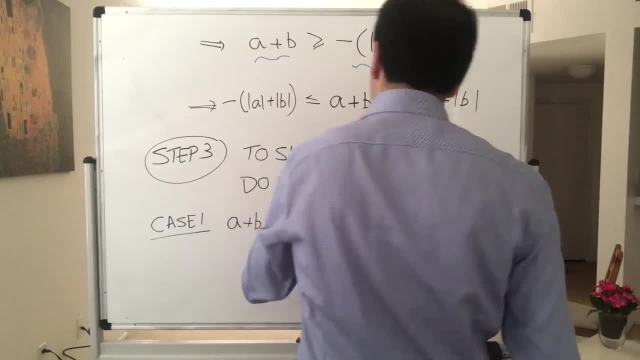 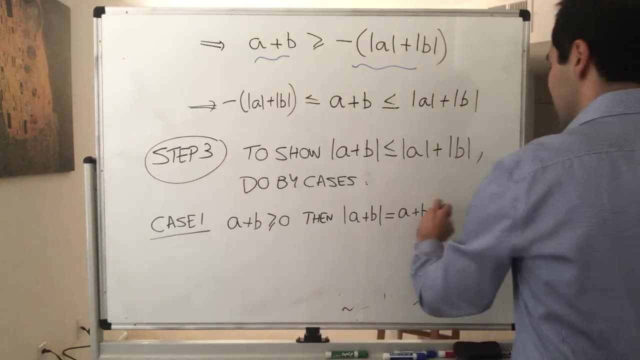 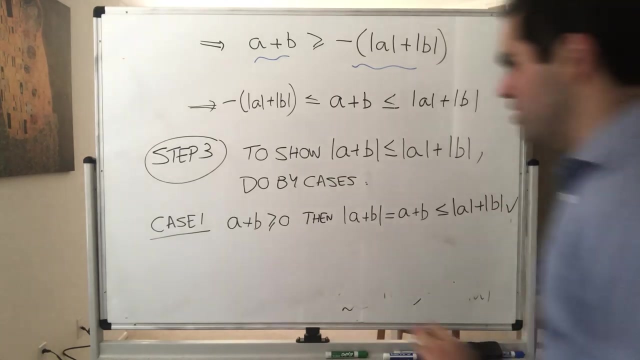 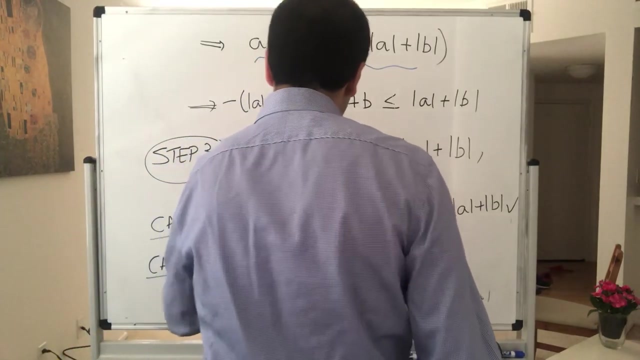 then what do we know? absolute value of a plus b, that's a plus b, but we know this is less to equal to absolute value of a plus absolute value of b. so in that case we're done. in case two, if a plus b is negative, then absolute value of a plus b is negative. then. 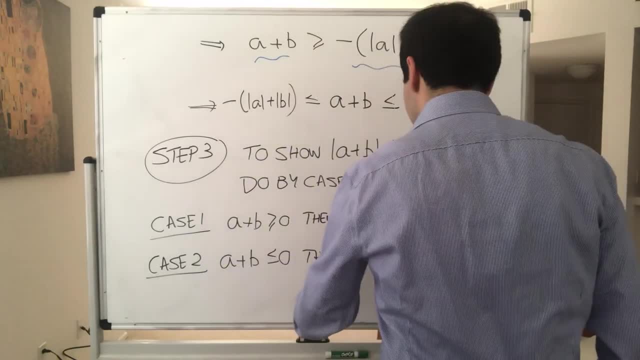 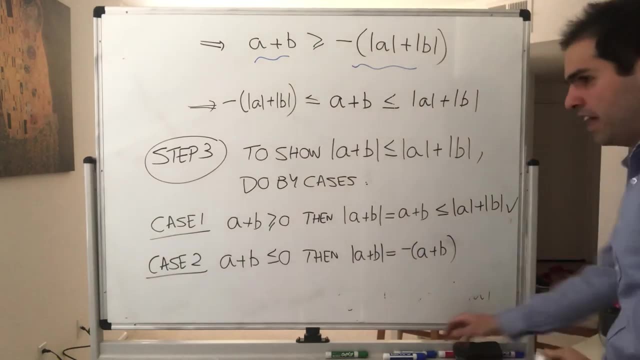 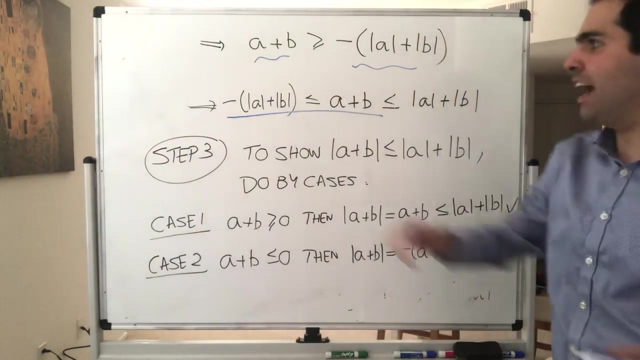 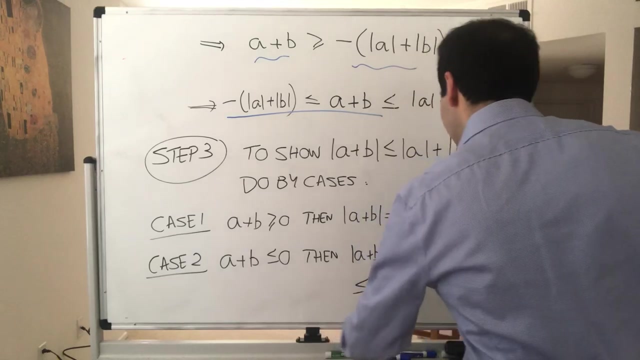 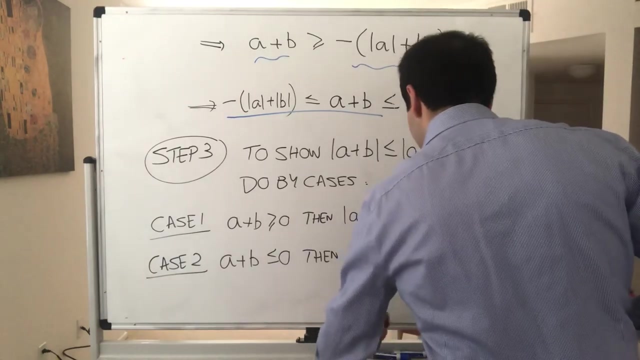 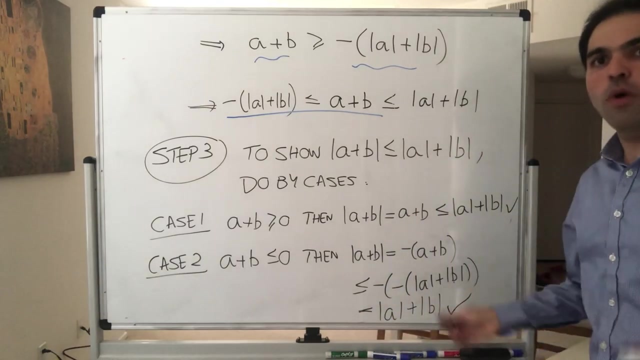 absolute value of a plus B. it's minus a plus B, but look then you just use this identity. you see a plus B is greater, equal to minus that. so minus a plus B is less than or equal to minus minus a plus E, and that's also a absolute value of a plus absolute value of D. in other words, in both cases. 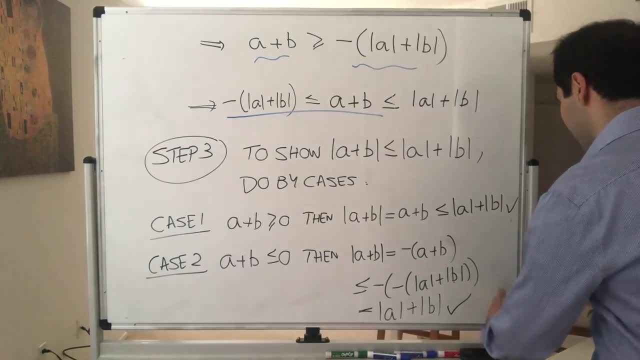 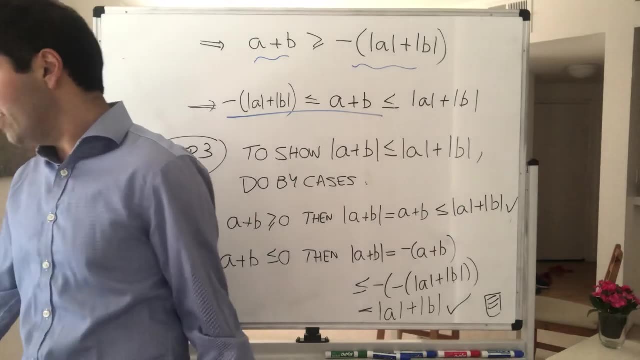 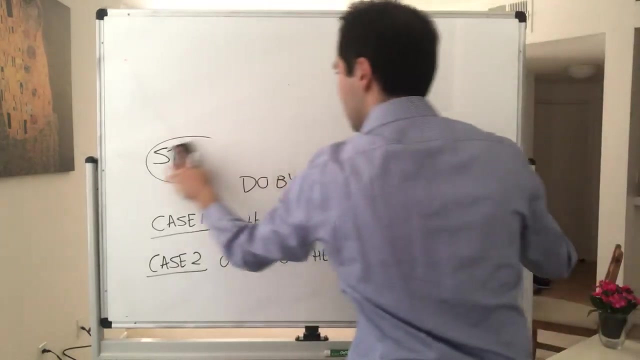 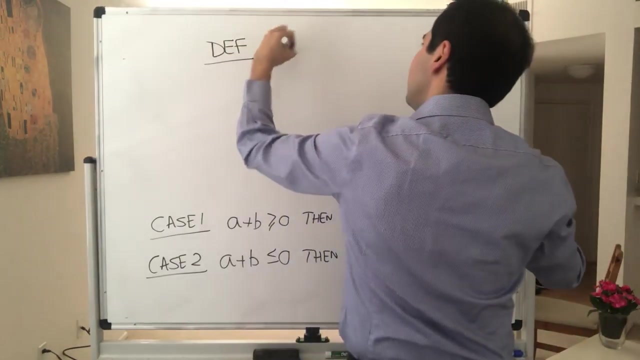 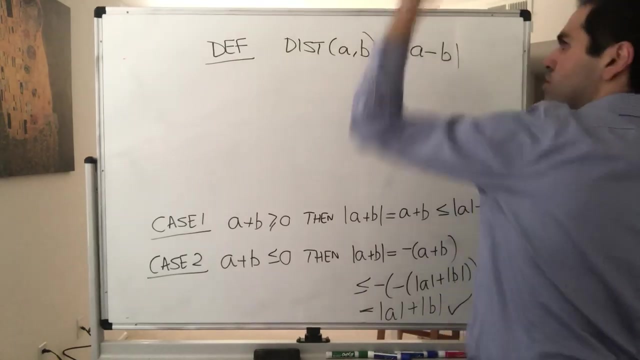 we have that, this is true and therefore we're done. that's but not least, why is it called the triangle inequality? well, it'll be clear after the following result. so first of all, just a little definition: the distance between a and B, that's absolute value of a minus B, also same as absolute value of B minus a, and it's literally the distance between: 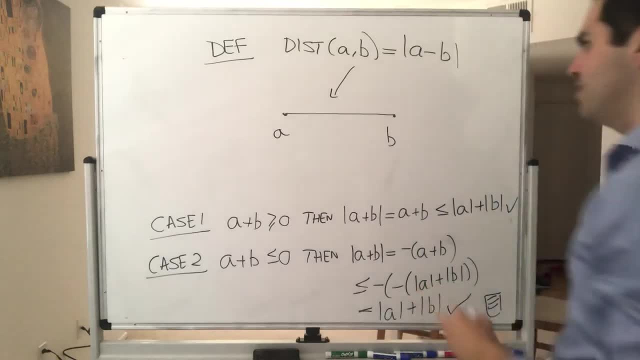 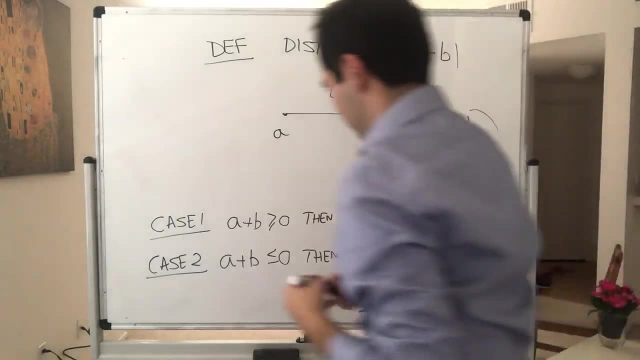 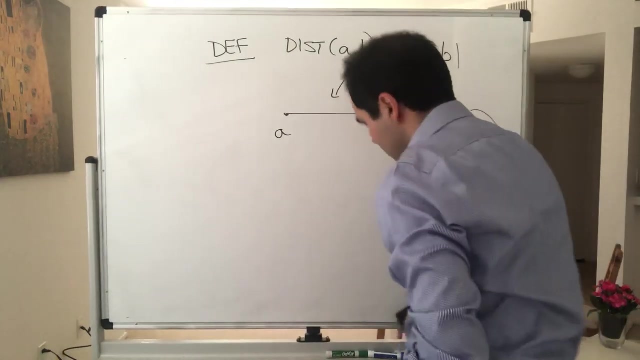 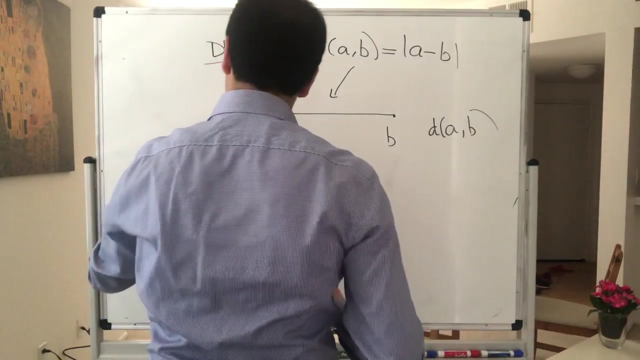 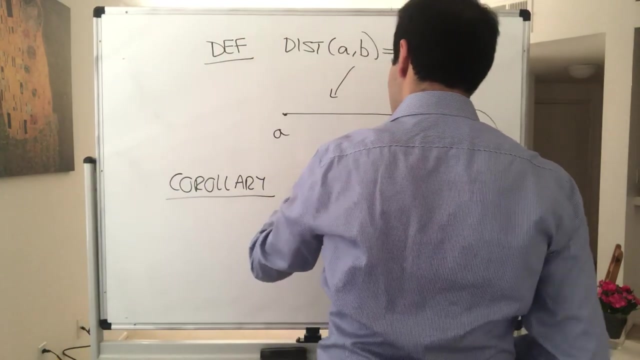 two points. and, by the way, some people- and we'll use that later- call it dab. and now what do we want to show? let's show the following again: so little corollary, so Toyota corollary. in other words, let's show that the distance between a and C it's less than or equal to the distance. 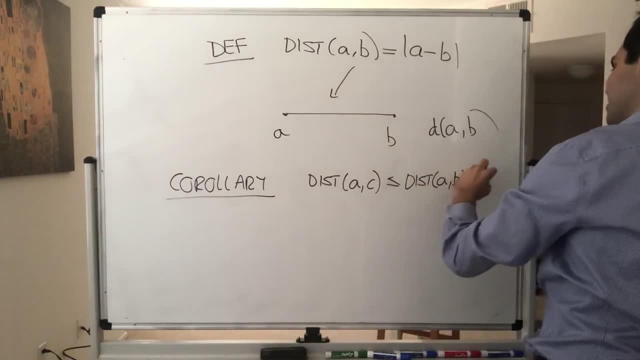 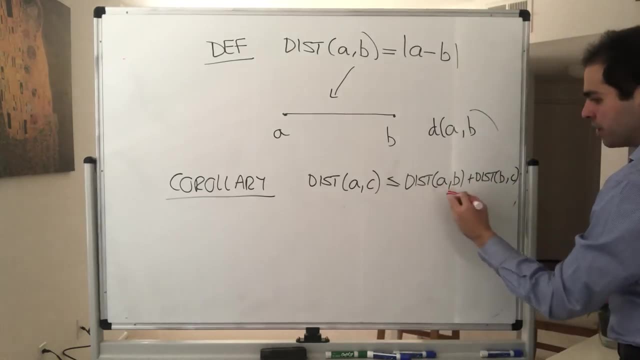 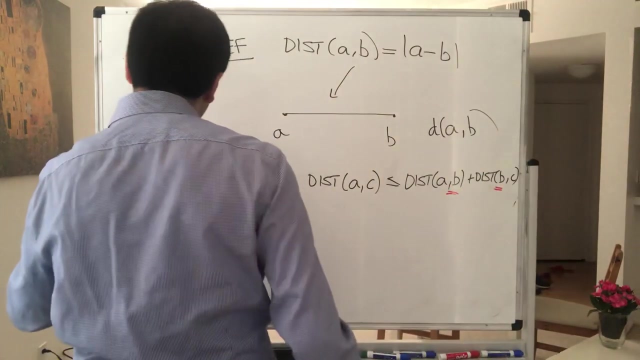 between a and b plus the distance between B and C. It's very important. In other words, you can add a B here, provided that you put a less than or equal sign, And the proof in my opinion is very important. So, because it uses an analysis trick we'll use over and over again. So 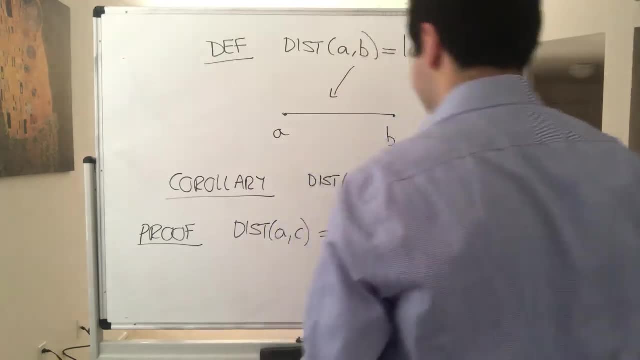 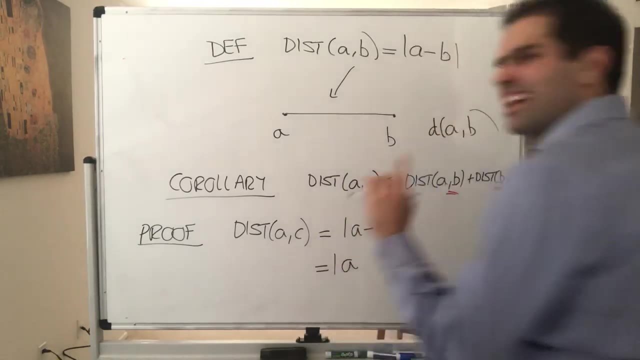 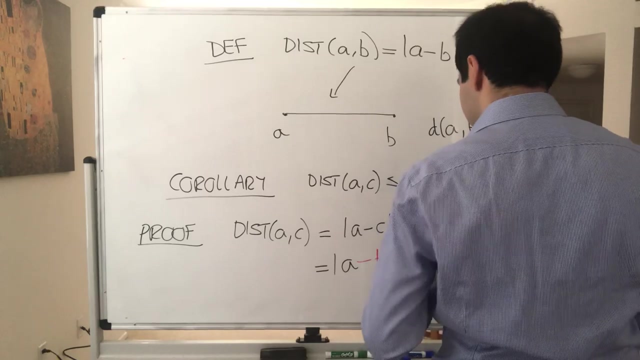 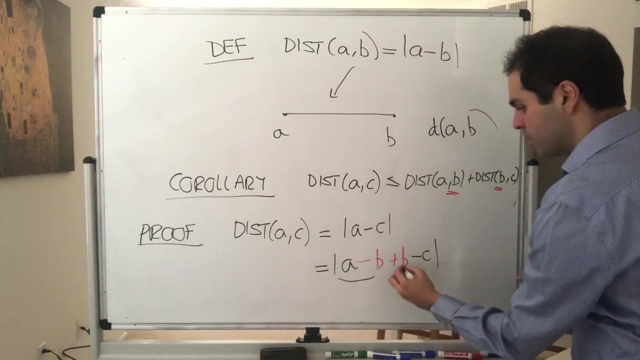 the distance between A and C. by definition, absolute value of A minus C. But now again, extremely important, We will use this over and over again: Subtract and add B. That's good, because now you have the sum of two things. So 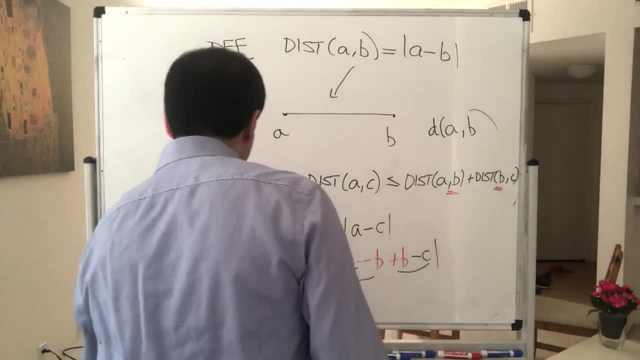 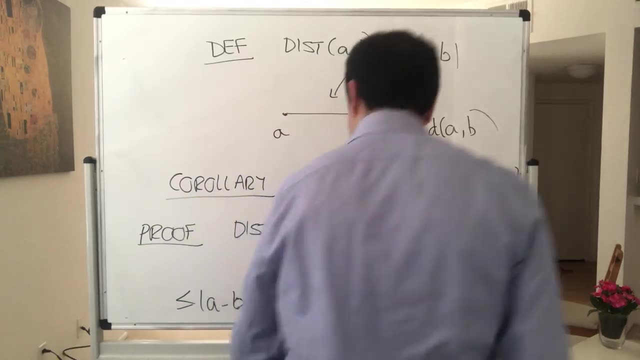 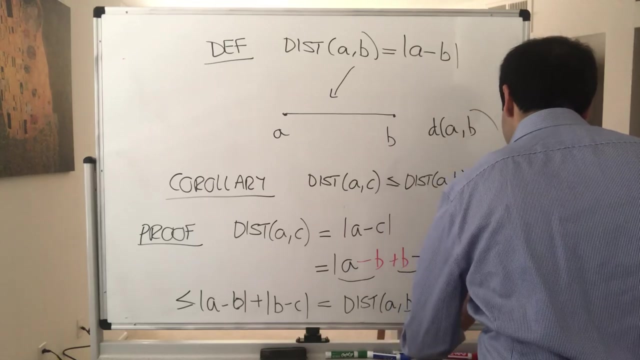 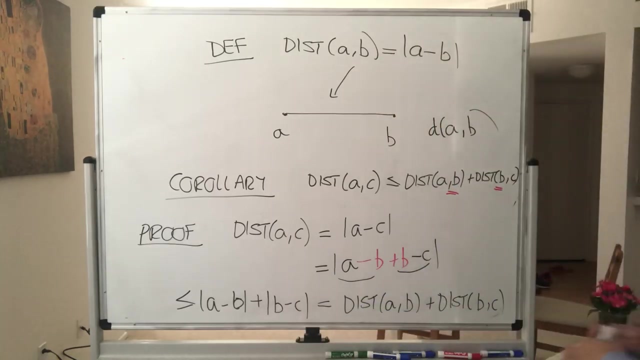 you can use a triangle inequality, So this less than or equal to A minus B plus B minus C, But by definition that's just a B, So the distance between A, B and the distance between B C. Okay, wonderful. And so this is done. And again, I like this because it really 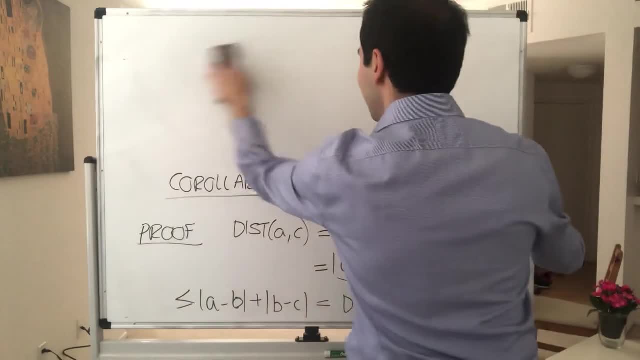 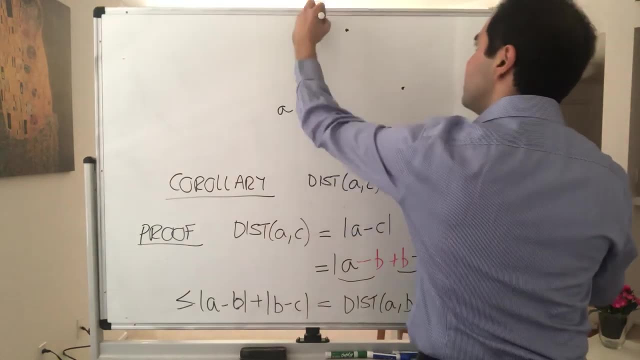 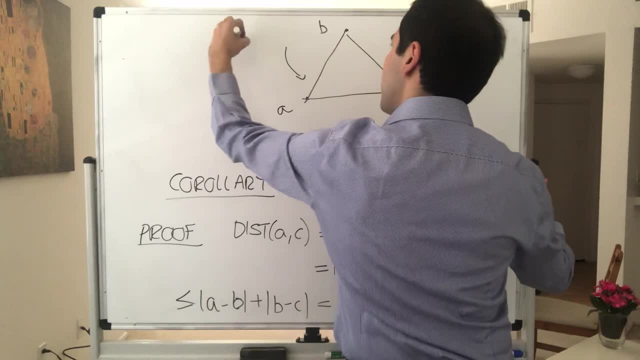 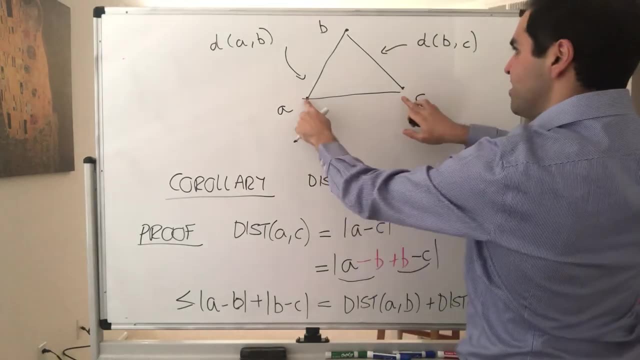 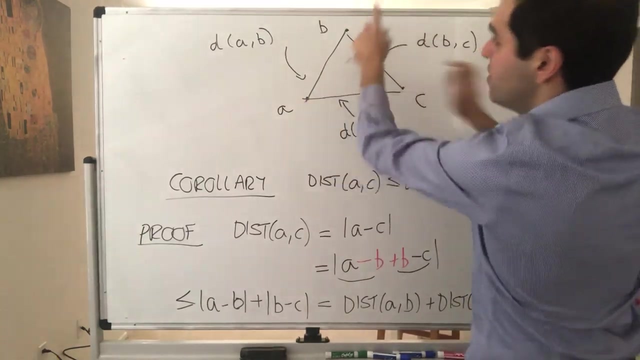 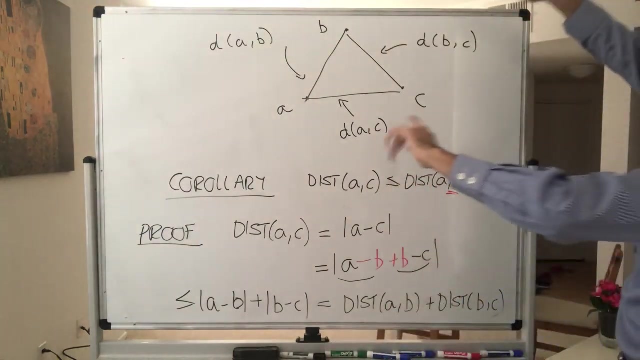 You see, this is the distance between A and B. This is the distance between B and C, And what this is saying is that this length, so this distance between A and C, is always smaller than the sum of the lengths of the other edges. So, in other words, the third. 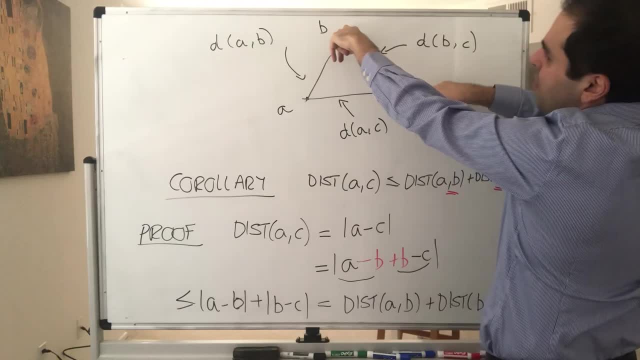 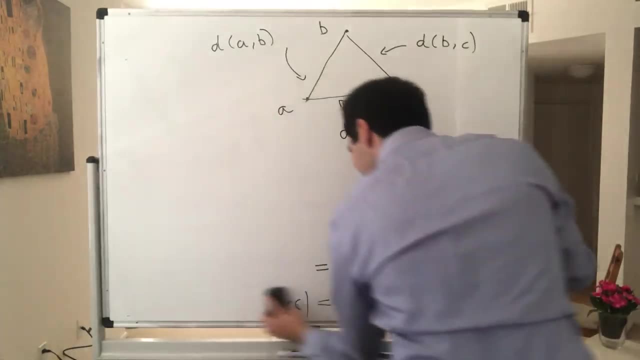 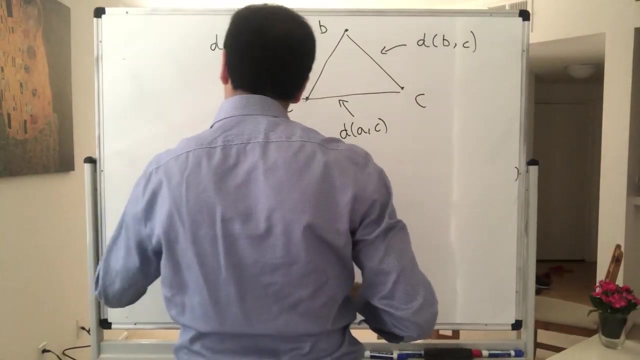 leg of a triangle is always less than or equal to the sum of the other two legs of the triangle. Last but not least, I would like to conclude with a related inequality which you can show in your homework, but that's called the reverse triangle inequality. 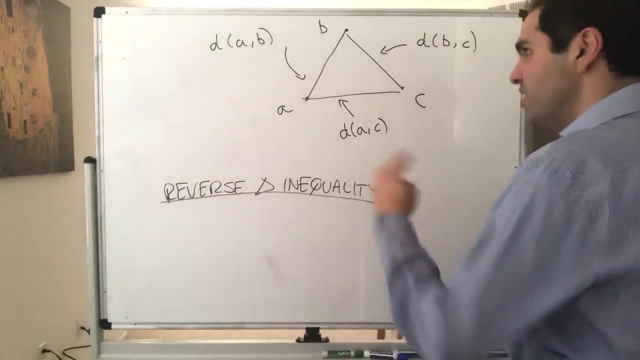 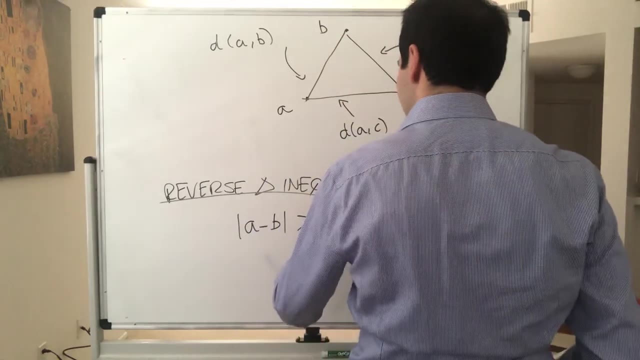 Because what's nice here? it goes less than or equal. but there's another inequality that goes like greater than or equal and it says the following: The absolute value of a minus b, it's greater or equal to the difference of absolute values. 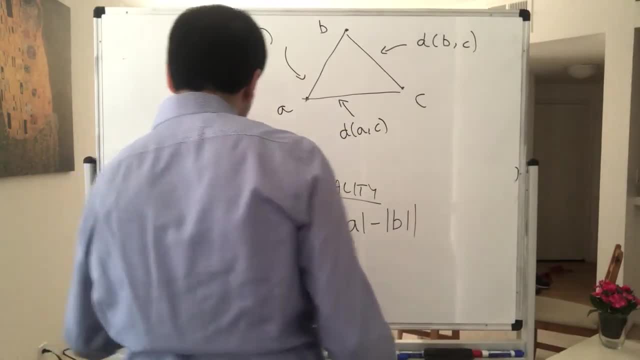 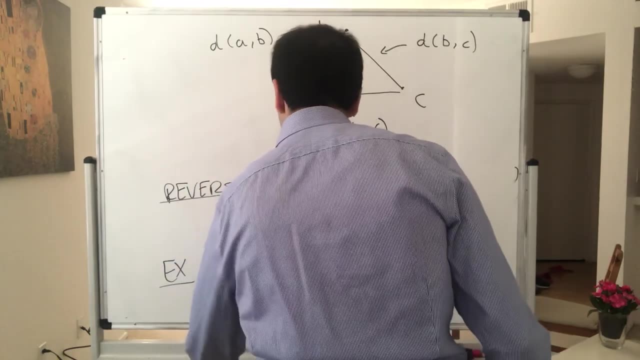 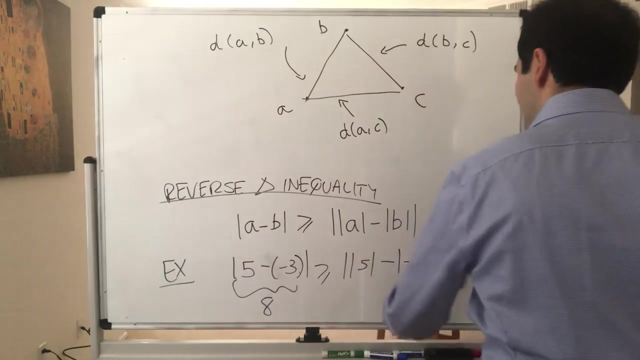 For instance, let me just illustrate: Take five minus minus three again, which is eight, and that's greater or equal to the absolute value of the absolute value of five, 5 minus absolute value of minus 3, which is 5 minus 3, and that's just 2..